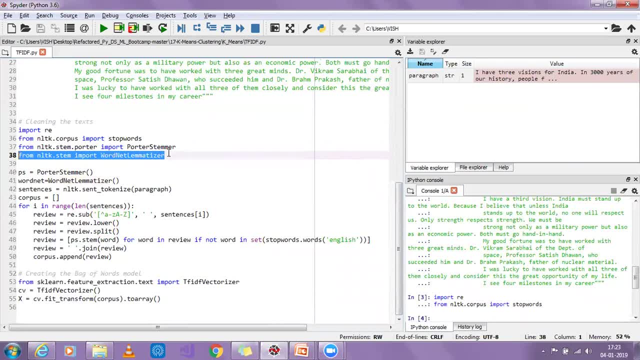 I'm just going to import word net lemmatizer, which is for lemmatization. So here it is. I've executed. You can see that my laptop is super fast. This thing executed very quickly. Okay, Then, once I've imported word net lemmatizer. 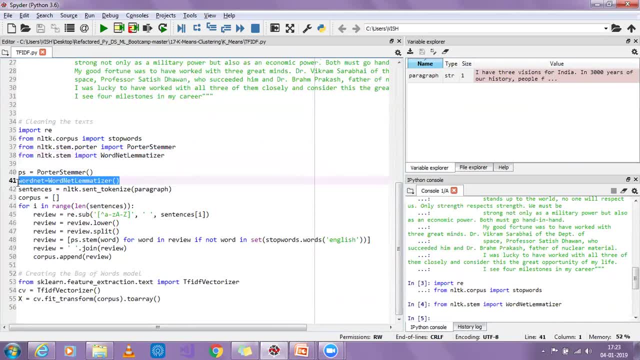 what I'm going to do is that I'm going to create a word net lemmatizer object which will do the lemmatization function. Okay, Now I have my paragraph. Always remember, I have to tokenize this paragraph, basically convert this paragraph into sentences. 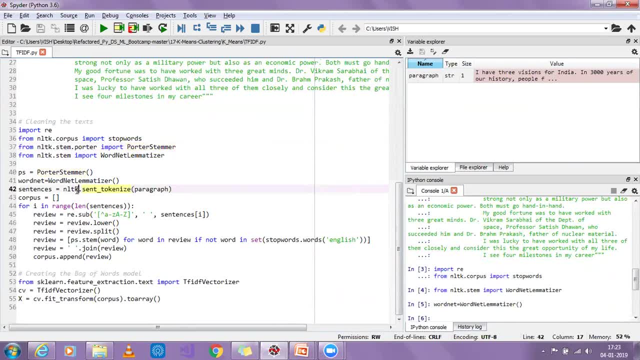 So I'll be using, I'll be using, I'll be using sent underscore tokenize function, which is present inside NLTK, And I'll convert my whole paragraph into sentences. Here it is. I'll execute this Now let us see that. how many different sentences I have. 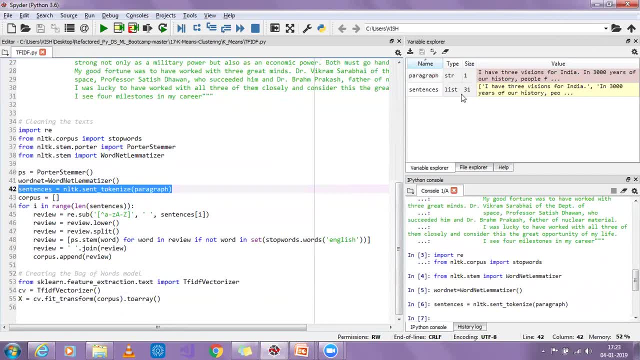 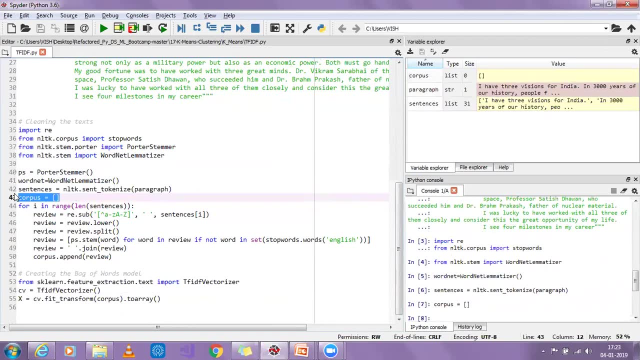 I have around 31 sentences, right? So this is my 31 sentences. Then I'm going to create a new variable, which is a new list, which is corpus, because I'll store everything from this paragraph after applying, you know, after removing the stop keywords and after applying. 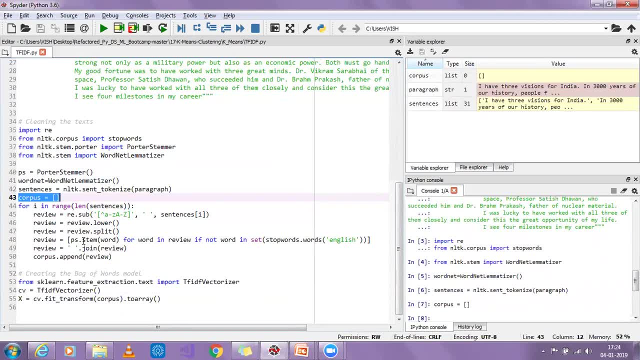 the word net lemmatizer, basically after doing the lemmatization thing. So what I'm going to do is that this statement is almost the same that we have discussed for the cleaning process in my previous video. If you have not seen that, go behind and see it again. I'll try to explain you. 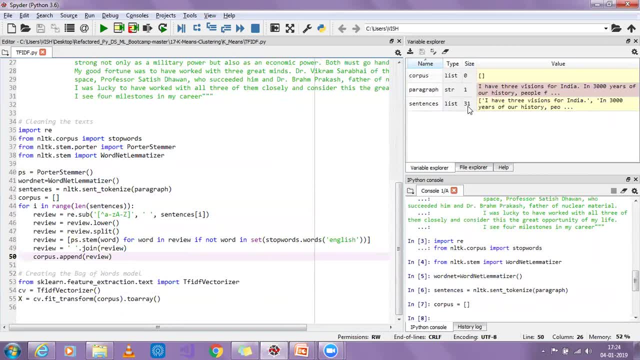 I'm going to put a for loop on all the sentences That is the size of 31.. When I'm putting the for loop, what I'm going to do is that this for loop will run from zero to 31.. So, basically, 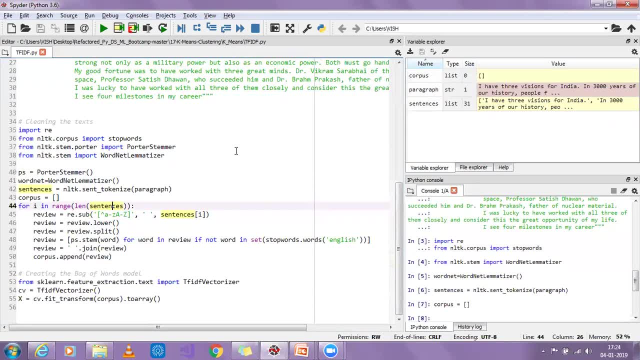 all my sentences. it will run with a range of all my sentences. So, on each and every sentence, this particular loop will run. This resub re for regular expression. I am removing each and every thing from that whole paragraph, apart from A to Z, and 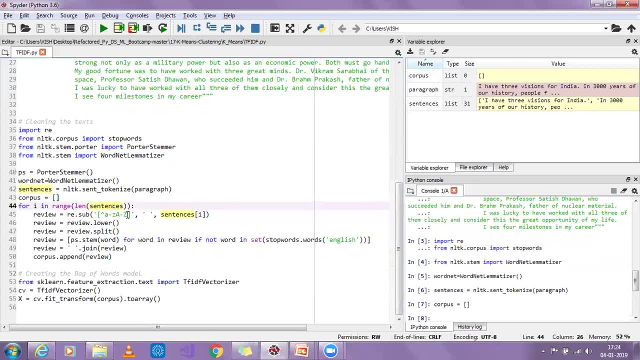 capital A to Z. Okay, I'm just cleaning up everything like full stop, comma, exclamation mark, question mark or any digits, because those will not actually play a better role in sentiment analysis. So I'm removing everything, Then I'm doing the lowering of all my sentences. 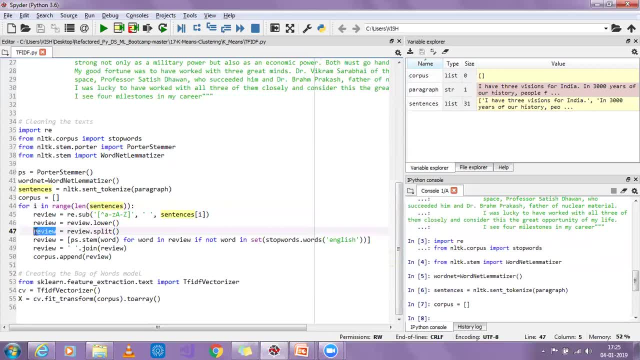 then I'm doing split of that sentences to get the split of words, I mean to get a list of words- then I'll apply a list comprehension. in this list comprehension I'll put a for loop for word in review. if not word, if that word is not present in stop words, I am going to apply, you know, word net. 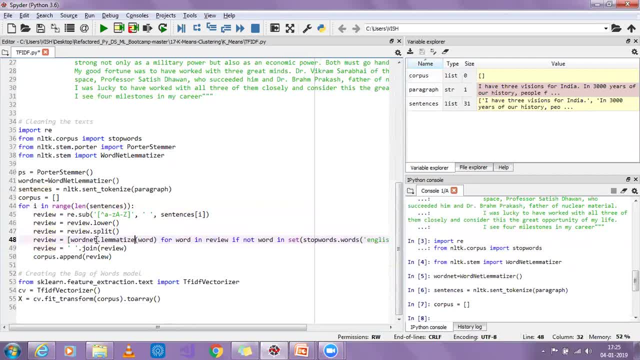 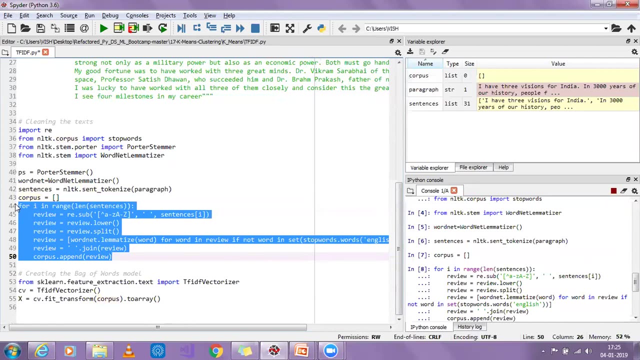 dot lemmatize. I'm going to do the lemmatization of each and every words and, finally, I'm going to join all the reviews that I have and append it in the corpus. so here it is. I have appended in the corpus. now let's see after executing this. it should get executed quickly. yes, it has got executed. 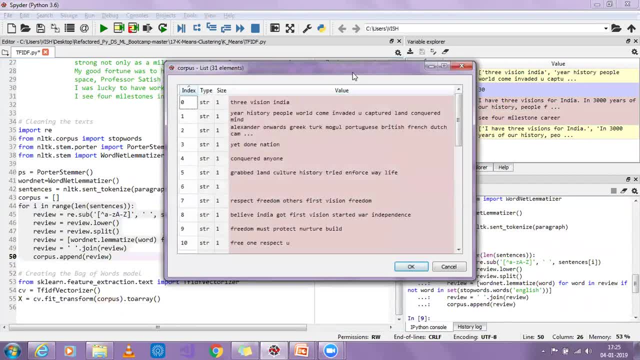 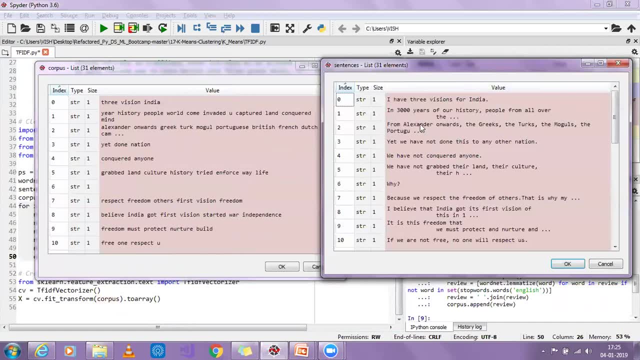 quickly. now let us do one thing. let us let us select the corpus and let us select the sentences. now let us compare it. okay now. the right hand side is basically my sentences, after applying lemmatization and removing the stop keyword. this is my left, so it has removed almost everything and it is looking a very good sentence altogether. 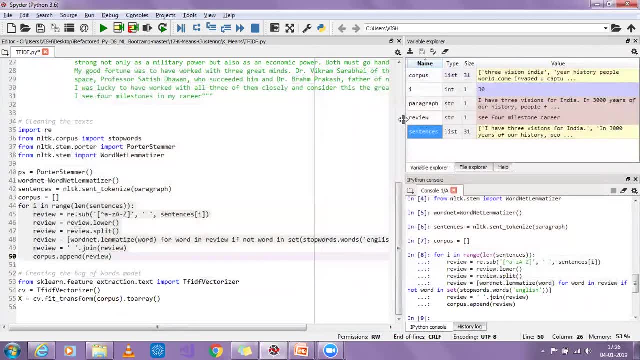 okay. now the next thing is that: how can i apply a tf idf model now in order to apply tf idf? i'll just remove this. there is not bag of words. i'll write it as tf idf. now, in order to create this tf idf, what i'll do is that i'll import a library which is called as tf idf vectorizer. 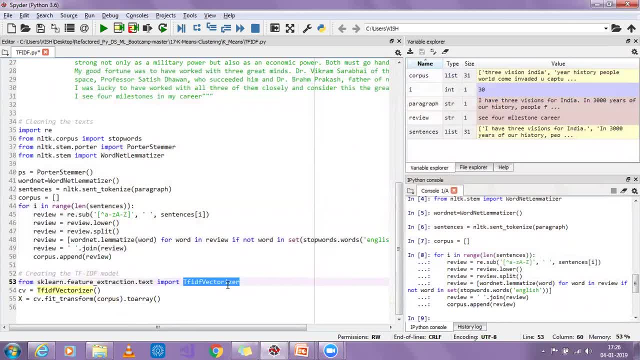 now remember, guys, for bag of words, we imported something called as count vectorizer, but for tf idf, i'll upload a library which is called as tf idf vectorizer, which is present inside sklearnteacherextractiontxt. okay, it is present inside skykit: learn library. 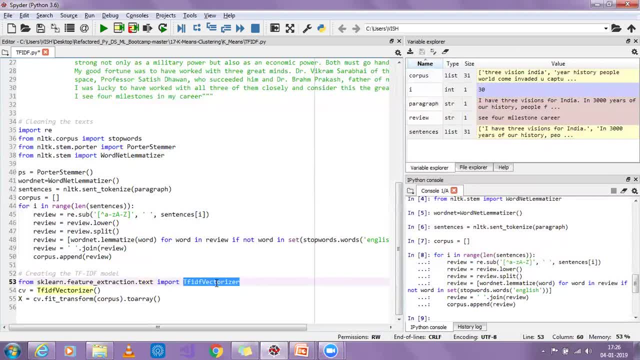 we'll import this library, which will be helping us to do the tf idf mechanism. then i'm going to create the object of tf idf, okay, and i'm naming it as cv and i'll write cvfit, underscore, tarp, tarp, transform for for this list of words and i'll convert this into tf idf. document matrix and 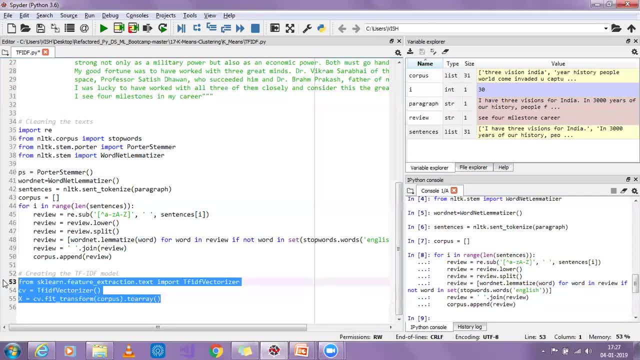 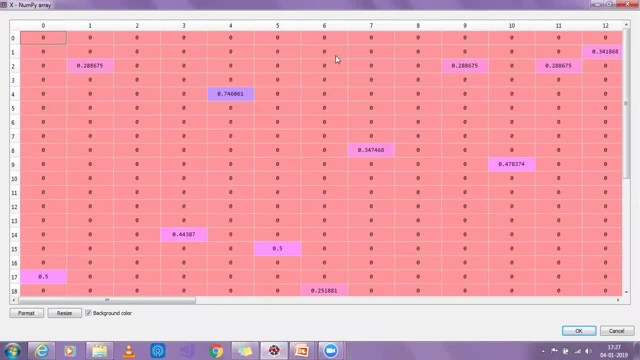 convert finally into an array. now, as soon as i execute it, you will be able to see that. so here is my x. let me just show you in a bigger manner. now you can see that i'm having some decimal values, some some different, different values right now. this actually gives the importance with